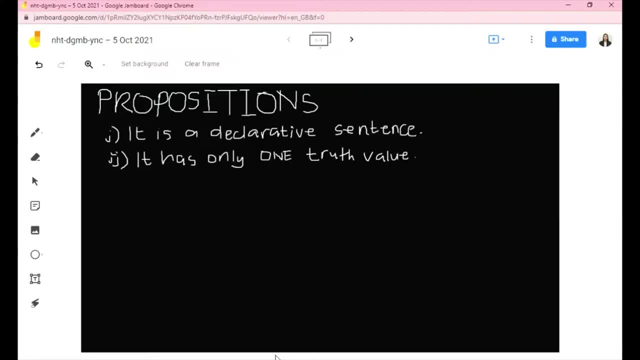 Okay, so good afternoon everyone. Let's talk about propositions. Propositions has only two conditions. The first one, it is a declarative sentence, And the second one, it has only one truth value. By truth value, we mean the truthfulness of the proposition. 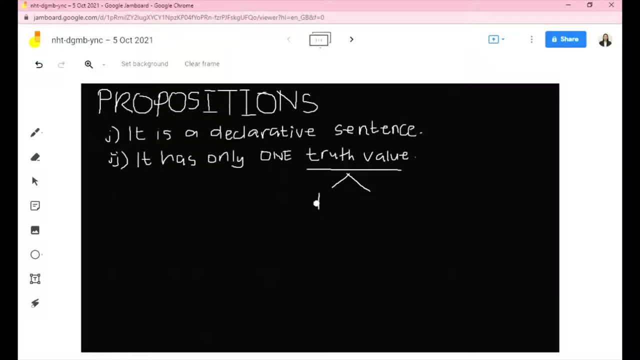 So we have only two options in here, whether it is true or it is false. Now for a sentence to be considered as a proposition, it should contain these two conditions: The first condition should be satisfied and the second condition should be satisfied also. 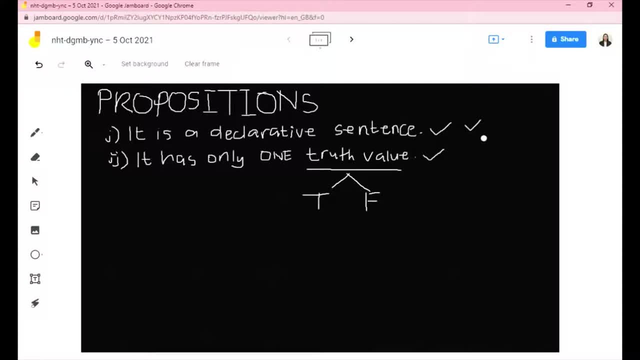 If the first condition is satisfied but the second condition is not satisfied, then it is not called a proposition. The two conditions should be satisfied. Alright, but before we continue on the propositions, I'd like you to introduce, or I'd like to introduce to you, the way of representing sentences. 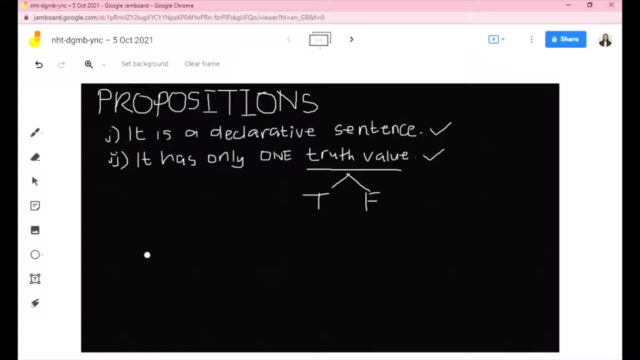 So we have two options: It could be in mathematical form and it could be in English form. For example, the mathematical form of the sentence X plus 1 is equal to 2.. Well, this is in mathematical form, but we can also write this one in English form. 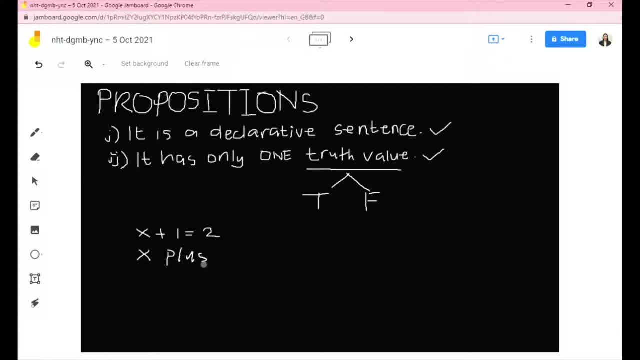 This becomes X plus 1 is equal to 2.. Alright now, aside from the mathematical form in the English form, we can also represent the English form into an argument form, or we can use propositional variables like P. So we will suppose that the statement P is our sentence. X plus 1 is equal to 2.. 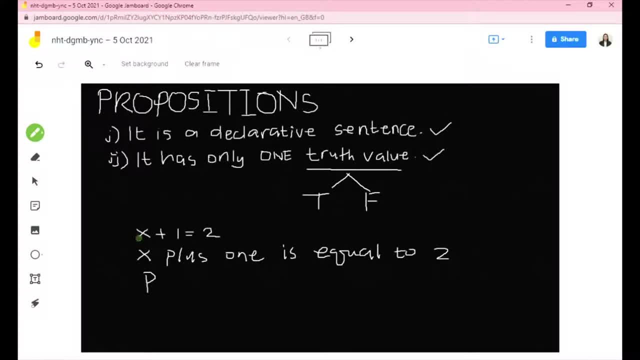 Now again, a mathematical form can be represented by using an English form, and an English form of a sentence can also be represented by an English form. It can also be represented by a propositional variable. Now let's continue on our topic. Let's try to identify if the following sentences are considered as a proposition: 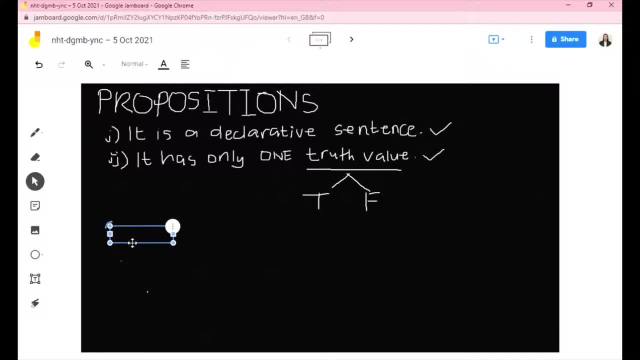 Okay, Let's have, for example, this sentence. Let's have the example. let me write it here: Hmm, 2 plus 1 is equal to 3.. 2 plus 1 is equal to 3.. Let's have the other sentence. 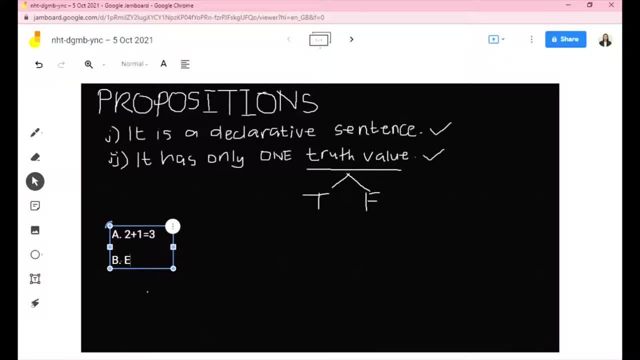 Emma is a pretty girl. Let's add another sentence. Let's say: are you hungry? And the other sentence: I hate you. Okay, so let's start identifying whether each of these sentences can be considered as a proposition. Now again, we only have two conditions for that. 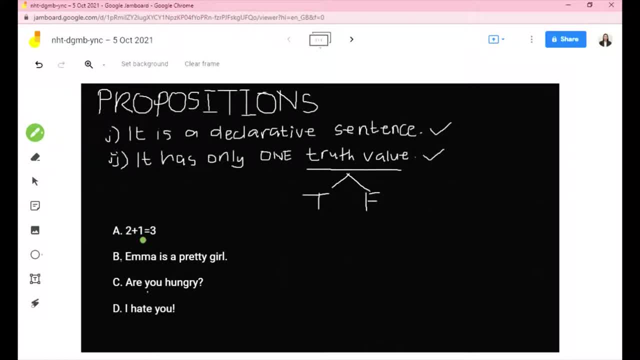 Okay, let's begin with the first sentence. 2 plus 1 is equal to 3.. Is it a declarative sentence? Now, what is a declarative sentence? by the way, We have different types of sentences: The imperative, the interrogative. 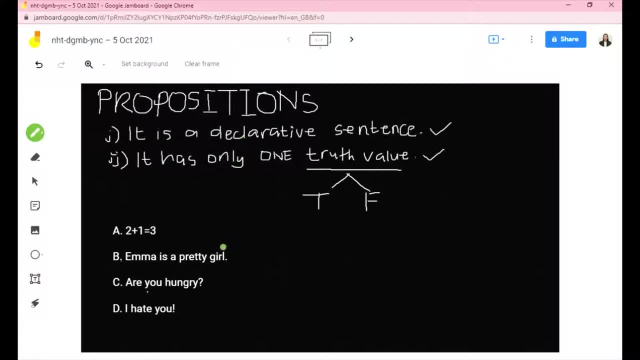 The declarative and the exclamatory sentence. So in this case, the first sentence is a declarative sentence. It states a fact, It gives us information about something. Now take note: if we will convert this mathematical form into an English sentence, we will have: 2 plus 1 is equal to 3.. 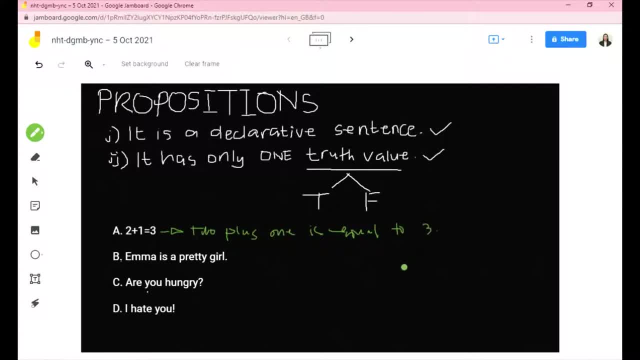 3.. So it is a sentence, a declarative sentence. specifically, It has a subject and a predicate. Now it satisfies our first condition. What about the second condition? Does it have only one true value? 2 plus 1 is equal to 3.. So let's try to solve that: 2 plus 1 is equal to 3.. On the left: 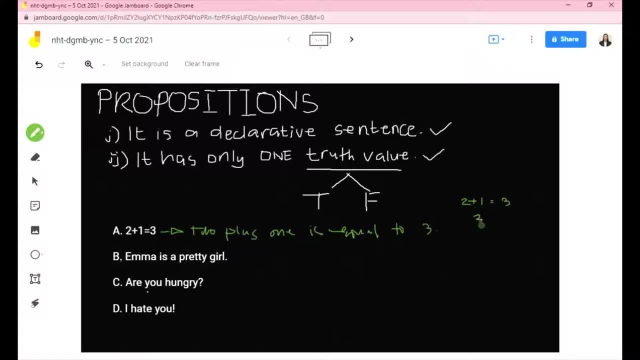 side, we'll have to add this: 2 plus 1, that is 3.. The same goes for the other side. So this means that statement A is a proposition and its truth value is true. Now let's have sentence B, Emma. 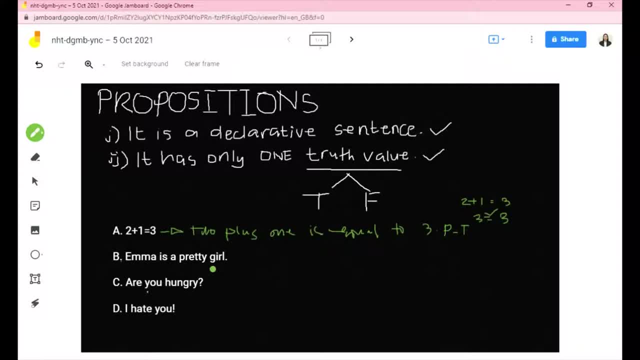 is a pretty girl. So let's see if it satisfies the first condition. Yes, it is a declarative sentence, But what about the second condition? Does it have only one truth value? So if you were to ask someone whether she find or he find? 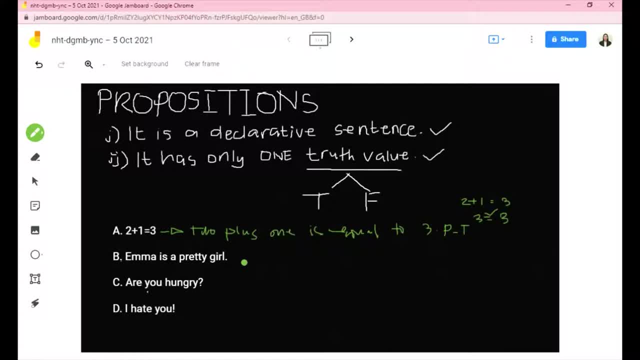 Emma as pretty, the other will probably say, yes, she is pretty, But the other individuals will disagree that no, Emma is not pretty. So there are two truth values: The true- for the others, it's true that Emma is pretty. The false for the others: they do not agree that Emma is pretty. And since this instance, 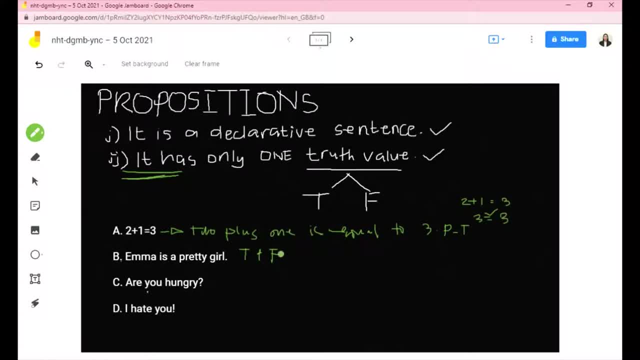 violates the second condition. therefore, it is not a proposition. Okay, it's not a proposition. Take note: this is subjective. What do we say by subjective? What do we mean by that? It's simply based on the emotions or the opinions of other people. 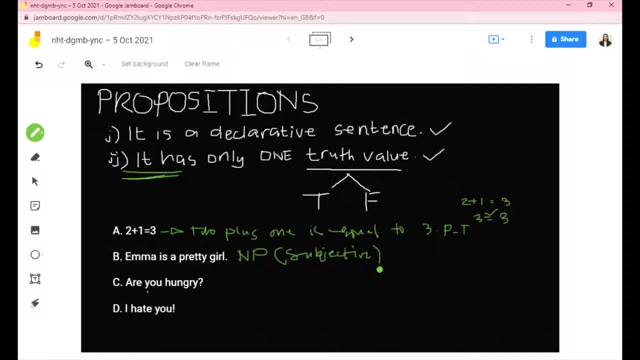 So it could be true to other and it could be false. for the rest, There are two true values. It does not satisfy the second condition. Now let's have statement C: Are you hungry? So let's consider this one. Are you hungry? It has a question mark. And if it has a question mark, 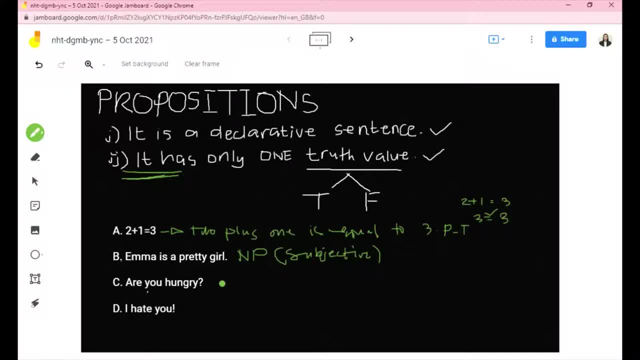 it is asking a question. If it is asking a question, then it is an interrogative. If it is asking a question, then it is an interrogative sentence. If it is an interrogative sentence, then it is not a declarative sentence. If it is not a declarative sentence, then 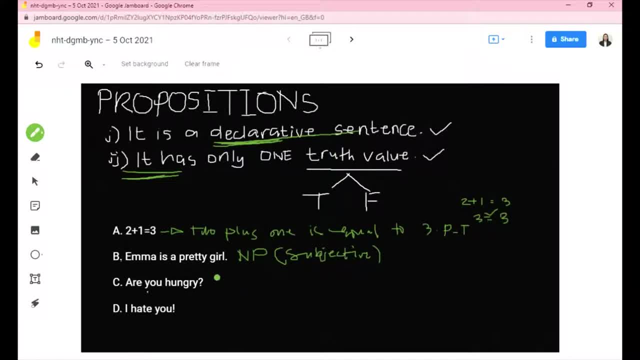 it does not satisfy the first condition. So this is not a proposition. Again, any of the conditions that will not be satisfied, automatically your example or sentence will not be considered as a proposition. proposition: now let's have statement d: i hate you. okay, let's see, this is a sentence, but it is not. 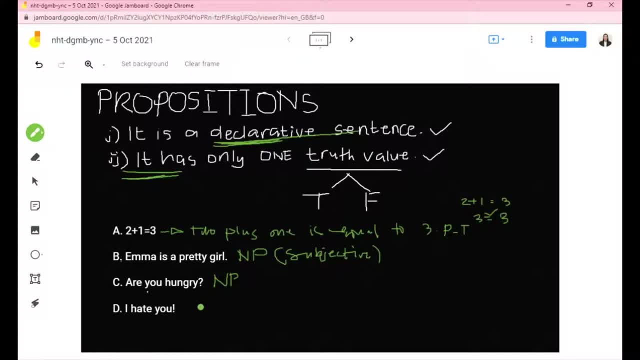 a declarative sentence. it is an imperative sentence, okay, no exclamatory sentence. rather, this is an exclamatory sentence, okay, so this is not a proposition. now, what if i have here- let's have another example, let me write it here- statement d. oops, let's have another example, statement e. 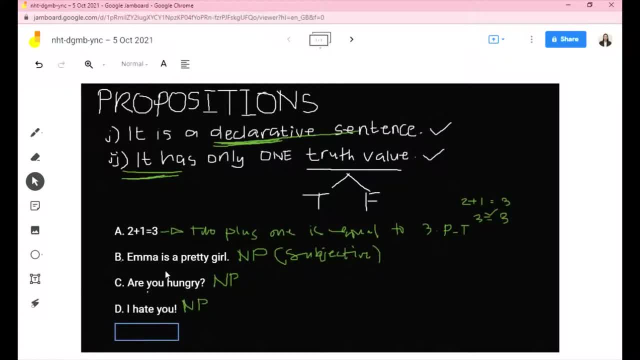 all right, e, x plus one is equal to three. and let's say we have another sentence here, statement f. let's say two plus three is just equal to five plus three. okay, so let's try to identify this sentence. e first: x plus one is equal to three. 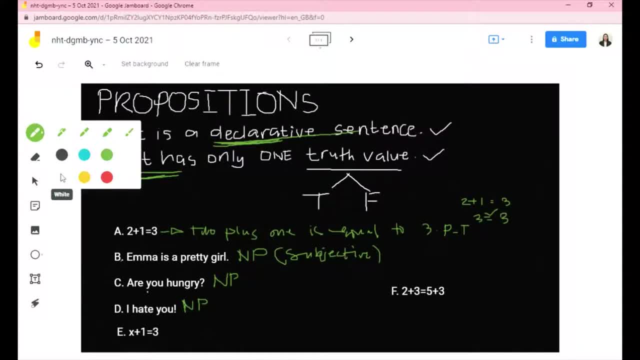 okay, x plus one is equal to three. this is a declarative sentence, so it satisfies the first condition. but for the second condition, remember it has only one truth value. it means there should be one truth value and it has only one truth value. so it satisfies the first condition. 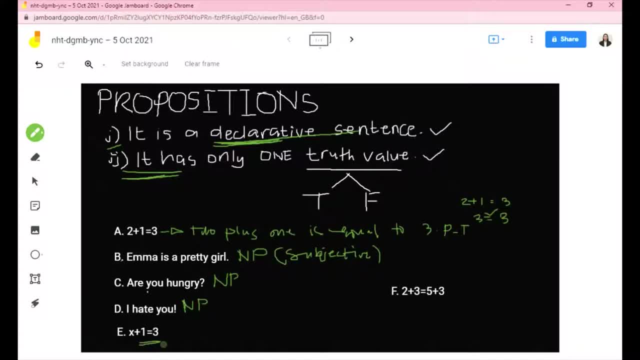 but in this case we cannot determine if the statement is true or false, unless or not, unless we have a specific value for x. so in this case it's not a proposition, because the truthfulness of this sentence depends on your value of x. so this will only be true if let's say, for example: 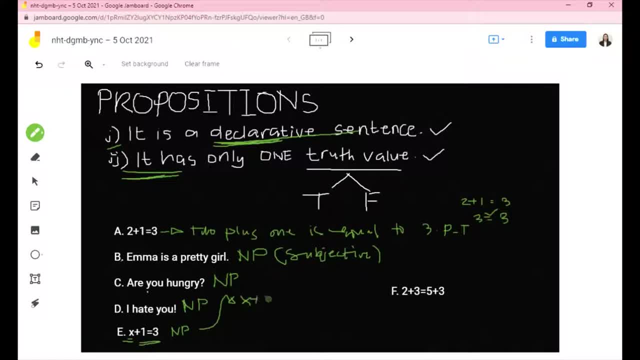 x plus three. let's say x plus three is equal to three, such that x is equal to x plus one, whether okay, x plus one is equal to three, such that x is equal to two. so substituting two to x will have: two plus one equals three. three is equal to three. so this can be a proposition and its truth value is true. or we can have: 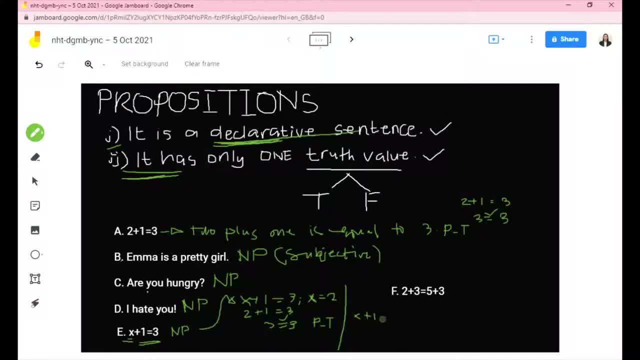 Like this: x plus 1 is equal to 3,, such that x is equal to 4.. Now we'll be substituting 4 to x. 4 plus 1 is equal to 3.. 4 plus 1,, that is, 5, equals 3.. 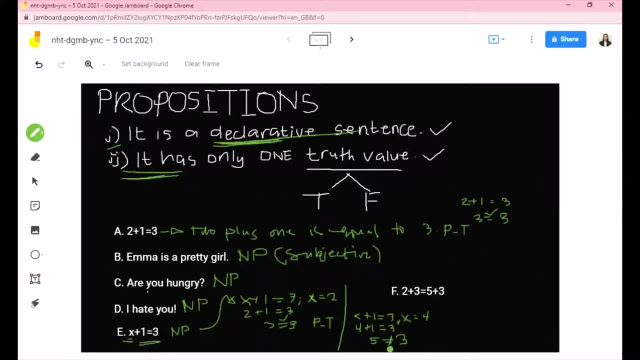 We know for a fact that 5 is greater than 3, so this is false. However, it can be considered as a proposition. So it's a proposition and its truth value is false. Now let's have the next statement, sentence F. 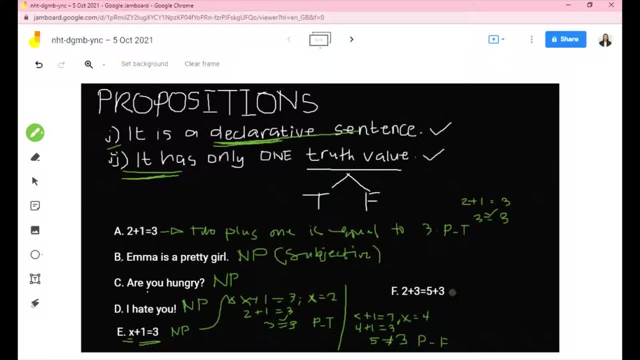 2 plus 3 is equal to 5 plus 3.. Now let's combine this: 2 plus 3,, that is 5.. Copy the equal sign and 5 plus 3,, that is 8.. This is a proposition. 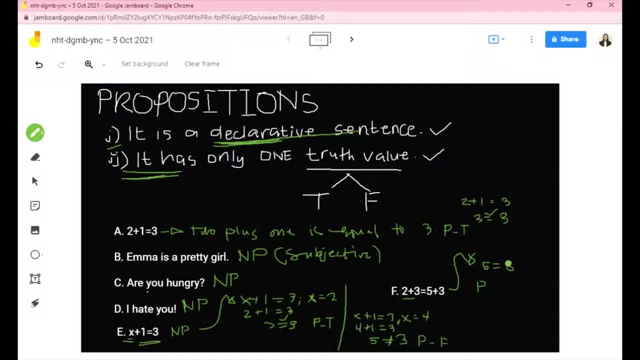 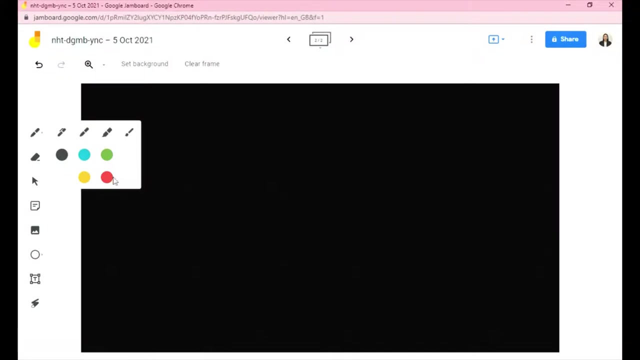 It satisfies the first condition, But it is false since 5 is not equal to 8.. So again, the main thought in here is just to satisfy the two conditions for your sentence to be considered as a proposition. Now in English we have also connectives that we usually use to combine two or more sentences. 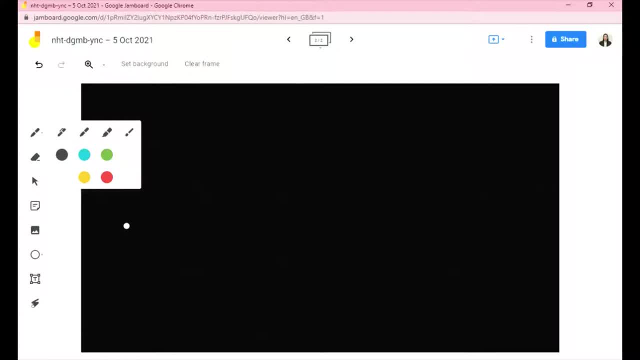 It's the same with logic. However, in here we will be using logical connectives. They're called logical connectives. Okay, So let me write it in here: Logical connectives. Now let's begin with the first one. 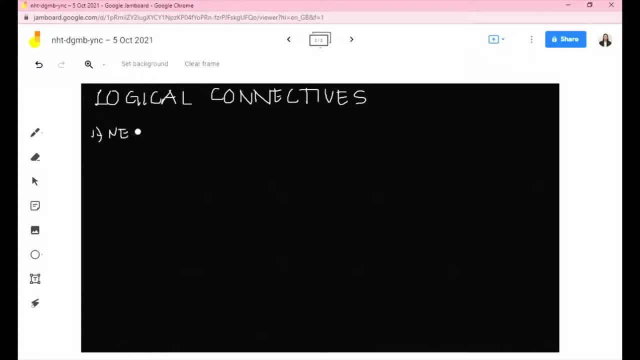 Well, let's start with the first one, first connective, that is the negation. okay, the negation is given by the symbol, this one, and it's read as not. so if I have here a propositional variable, P that represents my statement or my proposition, then the negation of P will. 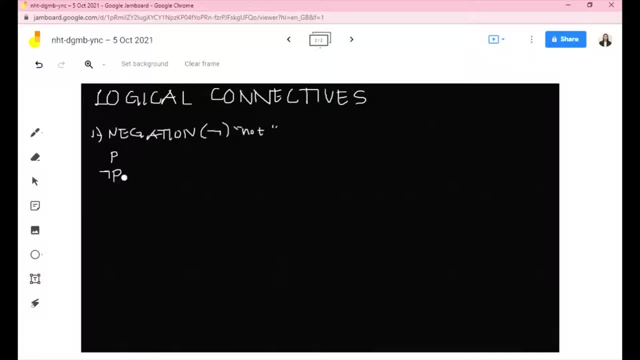 be not. so let's suppose that my statement P or my proposition P will be: 2 plus 2 is equal to 4. then if I will take out the negation of this particular proposition or the not P, it will be: 2 plus 2 is not equal to 4, so you'll only 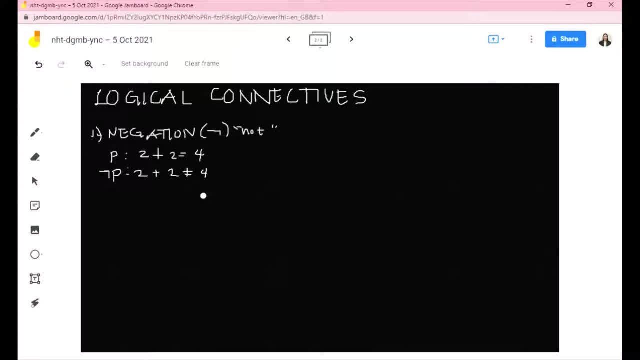 be writing. you'll only be writing the opposite, or the other way around, right, so you'll be contradicting your statement G. okay now how do we find or how do we look for, the truth values of the negation? let's consider the truth table in here. we only have one variable. 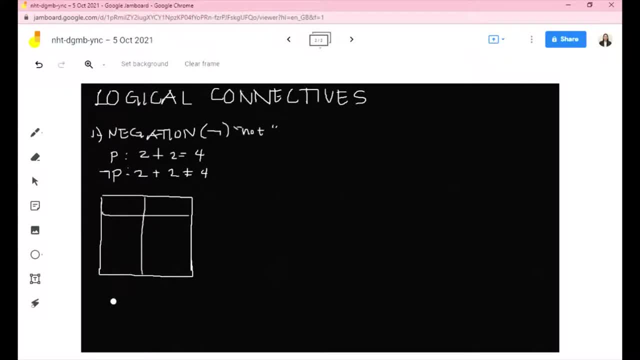 in here. so the given formula for that: how many rows will we be making for? In this particular example, we have one variable on me, so that's two raised to one or simply two. that means we will be making two rows. so for the two rows you will divide that as one, because therefore we'll simply be making for two. 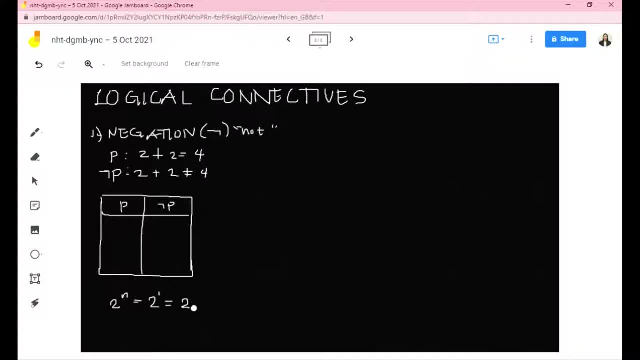 rows, but what we're going to do first is to write down what happened at the next line. we've been down to the largest point on the exponent side, just so. you mer sakho For the two rows. you will divide that into halves, or we divide this into two, then we'll have one. 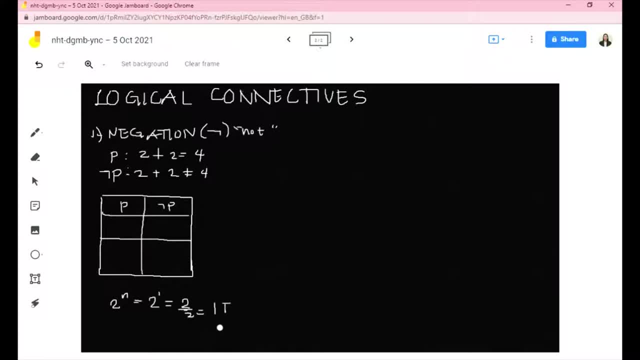 It means we start with one true, followed by one false. This will be your pattern: So true and false. Now take note again. we have mentioned: negation is just the opposite, or the not P, or the negation of P is just the opposite of your statement, P. 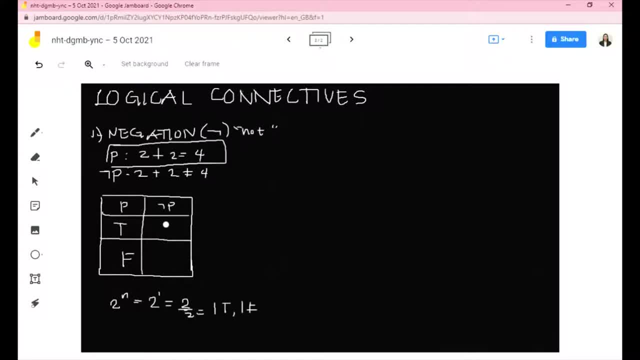 So if I have here true for P, then my not P would be false. If my P will be false, then my not P will be true. Now let's go on to the second logical connective. that is called conjunction. All right, let's write it. 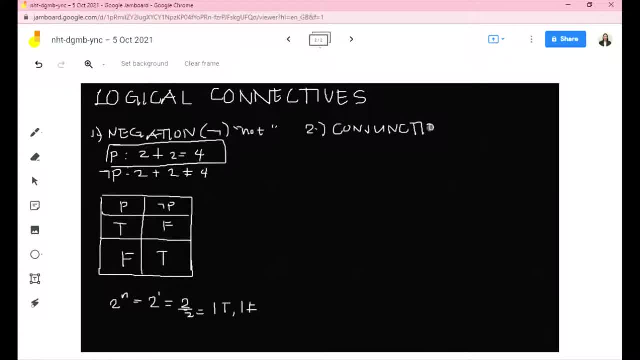 Here conjunction. The conjunction is given by this symbol. It's like an inverted V and it's written or it's read as: and in English: Suppose that P and Q are statements. Okay, if they are statements, once I use conjunction to connect these two statements. 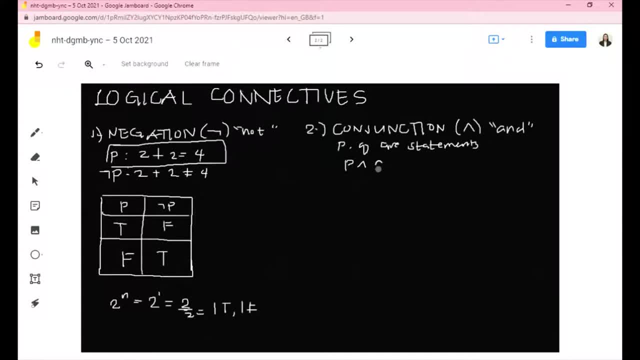 then I'll have P and Q. So if I have P and Q, then I'll have P and Q, Or you can read this as the conjunction of P and Q. Suppose that my statement P will be: it is not raining. 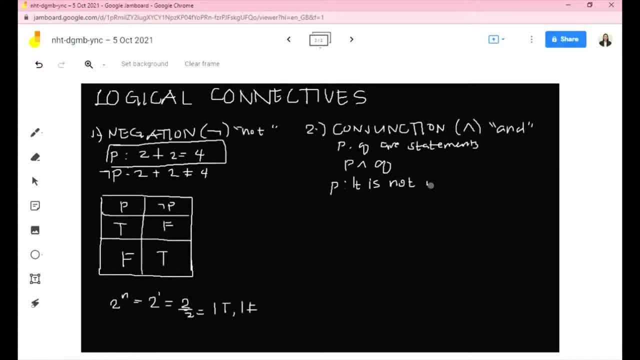 Okay, it is not raining And my statement Q will be- or my statement P will be, my propositional variable, Q will be my proposition. it is cold. It is cold. You might confuse yourself with propositions and statements, So they're just the same. 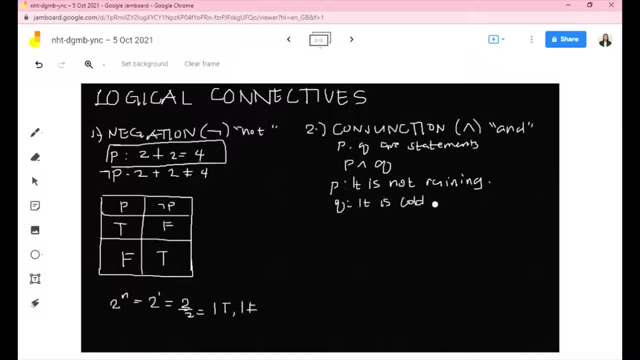 But in mathematics we usually call that as a proposition. Okay now, if I have here the statement P- it is not raining, And statement Q- it is cold, Then my P and Q will be like this: So our P. 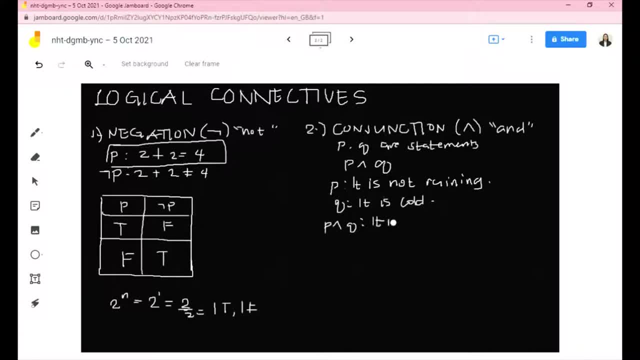 It's the statement: it is not raining. Let's just substitute: It is not raining. We have this symbol, conjunction in English, that is, and So we'll write down and in here, followed by our Q, which represent the statement: it is cold. 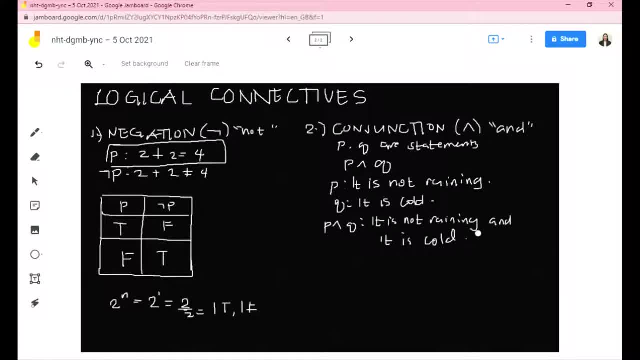 So your P and Q will be: it is not raining and it is cold. Okay, so we have P and Q. Now how do we deal with the truth values of these compound sentences involving conjunction? Okay, so for the conjunction it will only be true, or this proposition, P and Q can only be true if both P and Q are true. 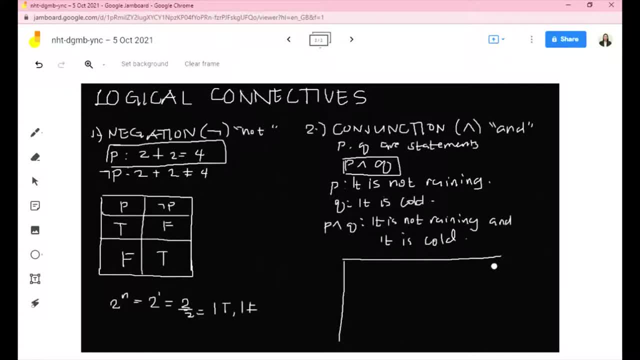 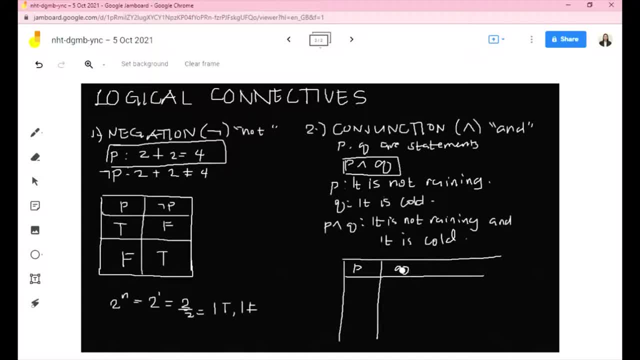 We have P and Q. We have P and Q. We have Q. This is for the second variable, And we have the compound statement P and Q. Now we'll have to see its truth values. How many rows will we be making? 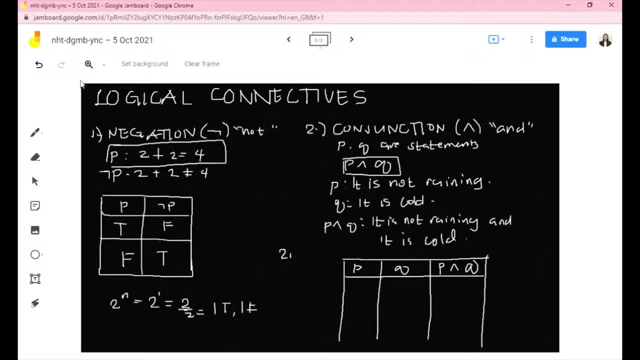 Again, use the formula 2 raised to n. That's equal to 2 squared. 2 squared because we have two variables in here, P and Q, So this gives us 4. It means we will be making 4 rows. 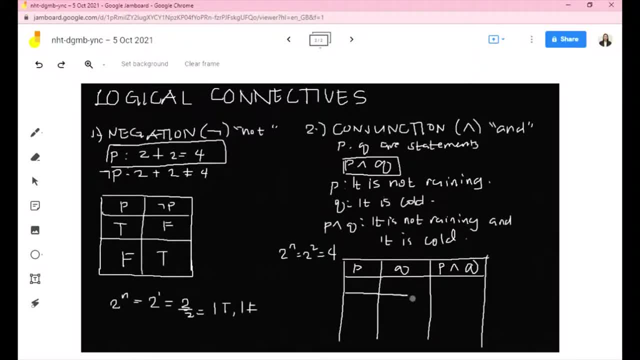 1.. Alright for a while. 1,, 2,, 3, and 4.. Okay, Now this 4,. we will divide this into 2 and we'll have 2.. So this means the pattern will be 2, true. 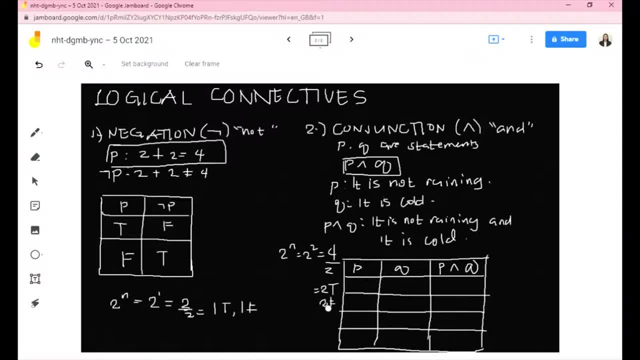 2 false. That is for the first column Right: 2 true and 2 false. Now on the second column, for Q, we have 2 in here, 4 divided by 2. That is 2.. Now the 2, we will be dividing that again by 2.. 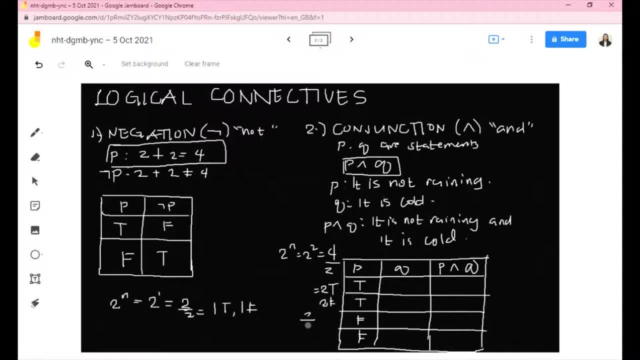 So 2 divided by 2. That is 1. Right, 2 divided by 2., That is 1.. So the pattern will be: 1 true, 1 false, 1 true, 1 false, 1 false, and so on. 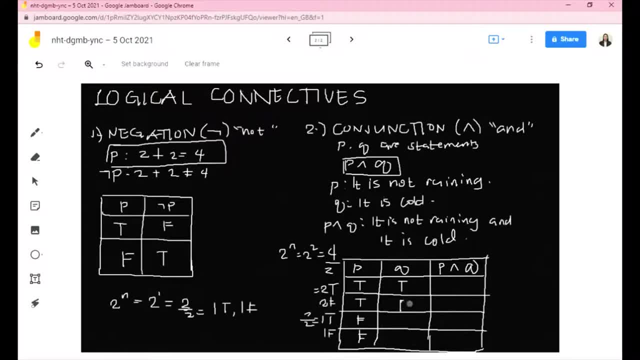 So this is true. This is false. This is true, This is false. Now let's go and get P and Q Again. P and Q will only be true if both your P, your Q are also true. So we have true and true. 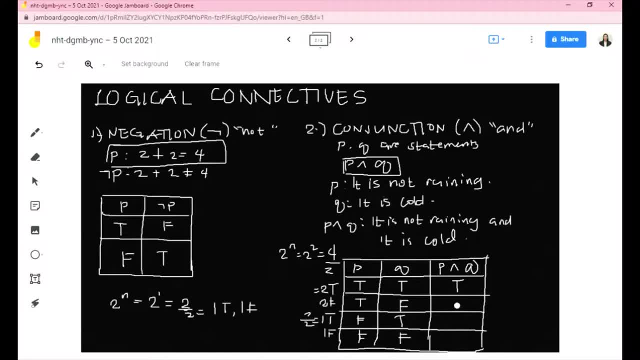 That is true. True and false: That is false. False and true: That is still false. And we have false and false: That's still false. So, you see, it will only be true if both of the propositions are true. 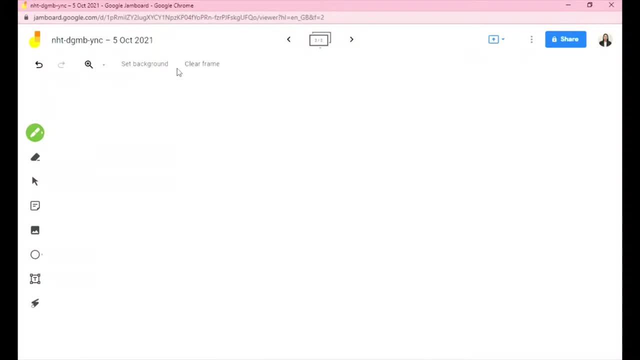 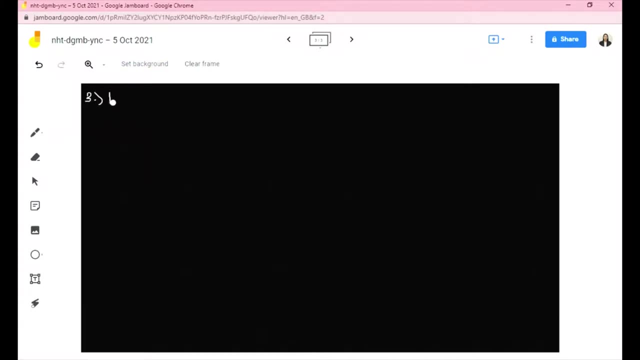 Right Now let's continue to the next connective Let's have here. the third logical connective is the disjunction. Disjunction is given by the symbol. it looks like a V, but it is a disjunction and it's read as OR in English. 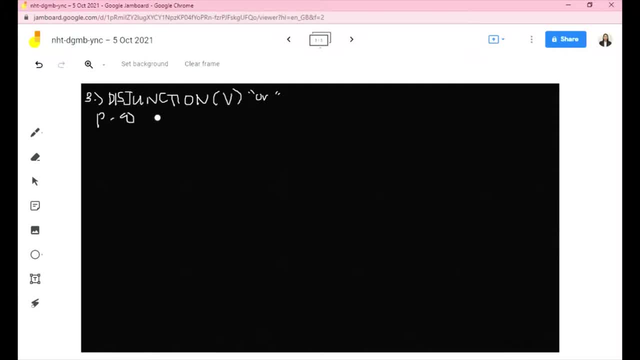 So suppose my P and Q are statements. If I will be using disjunction to combine these two statements, then my compound statement will look like this: P or Q. Alright, Now let's say that my statement P will be. It is raining. 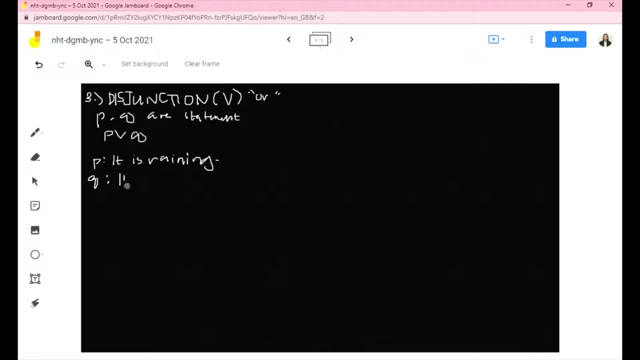 My statement Q will be: It is cold, So my P or Q, or the disjunction of two sound functions of p or q, will be like this: substitute the statement b, that is, it is raining, so we'll be writing that down. it is raining, all right, not, not a period, not yet. and then we have here this: 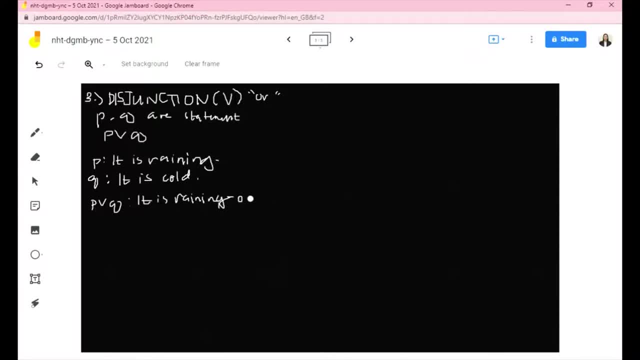 junction, or in english that's the word, or followed by your q: it is cold, it is cold period. so your p or q, or the disjunction of p and q is simply this sentence: it is raining or it is cold. now for the truth values, unlike for, that is, for the conjunction in, that is junction- p or q can be true when at: 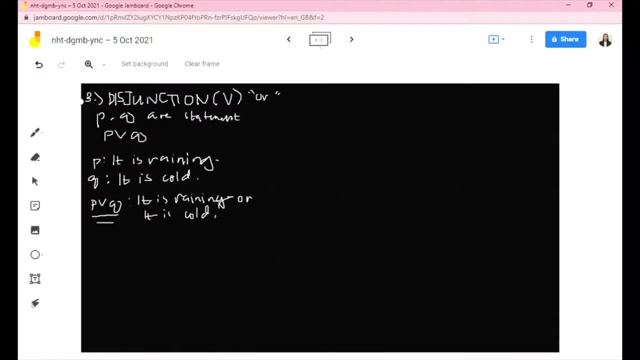 least one of the statements is true, otherwise it's false. so let's make a truth table for you to visualize it. okay, we have p, we have q and we have p or q in here, so we have two variables. that means we'll be making four rows, just like what we did for the conjunction. okay, one, two, three. 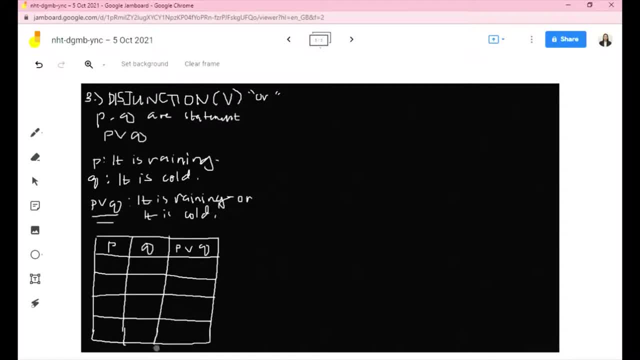 four: the same pattern: true, true, false, false, true, false, true, false. again for the p or q to be true, at least one of the statements or one of the propositions are true. let's have true or true. this is true. true or false. this is true. false or true. this is true. false or false. this is false. 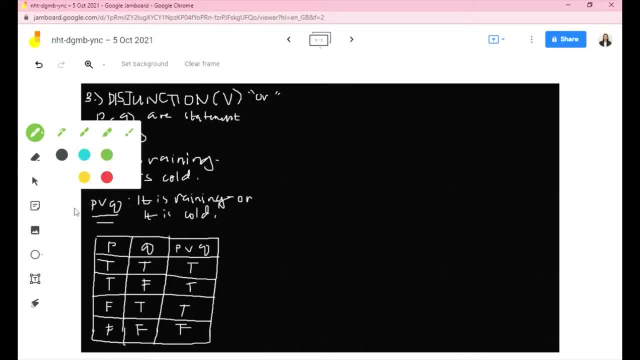 so you see, there is only one reason, or there can only one. there can only be one reason that will make your p or q be false. that is when both of your propositions e and q are false. now let's move forward. let's go to our fourth logical connective, and that is called the conditional. 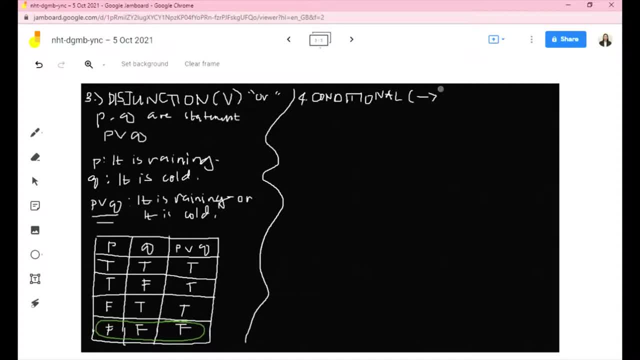 okay, conditional, which is in this form, and it can be read as if: then all right, so that is how a conditional statement is. suppose that i have here two statements, e and q. then my conditional statement will be like this: p implies q or p implies this. the parentheses Matrix, then the. resultado will be like this: you, if each one of these Ruby's error and based on the other, we get this argument that if p meets q, then the rest of the sentence will be just laufen and bench up by saying that toрен don't have to complain. to the first example and before you. 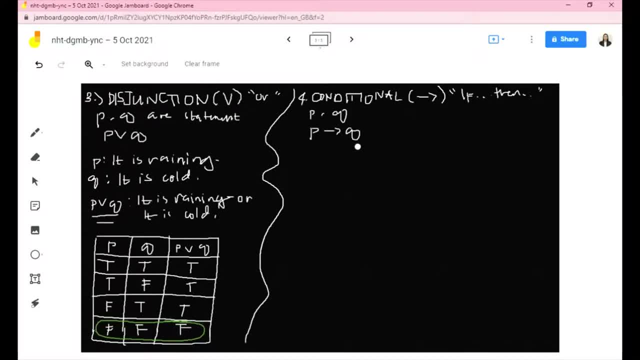 f, p, then q. so p here, this is our hypothesis, or antecedent. q here, this is our conclusion, or consequent. now for the conditional statement. it can only be false when your p is true but your q is false, so this will imply that your p implies q is false. again, in this case, there can only be 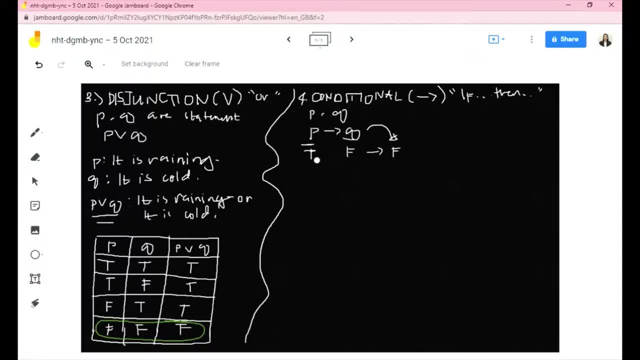 one reason for it to be false, and that is when your p is true, your q is false. otherwise it will be true. now let's start making a truth table right for a while. i'm having a trouble drawing a straight line here. so we have b, q and p implies q. now we still have two propositional variables here, so we'll have four. 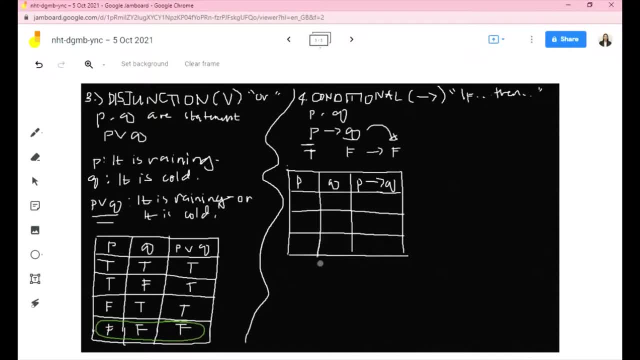 rows again and the pattern continues. the pattern is just the same same: t, t, f, f, t, f, t, f. so let's start. don't forget: this is the only reason that your p implies q will be false. okay, t implies t, that is true. t implies f- right, it's the same with this case. so 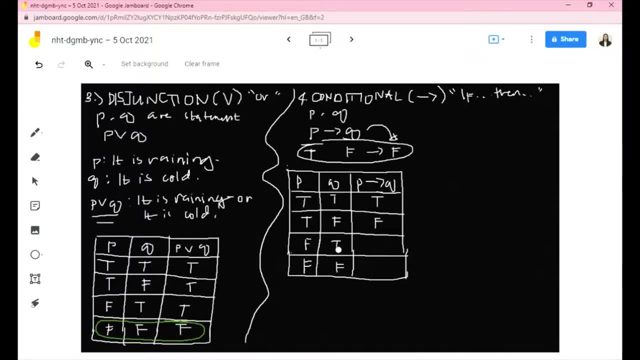 it is false. false implies true, that is true. and false implies false, that's still true. now you see, there can only be one reason for your p implies q be false, and that is when your antecedent is true, but your consequent is false. now for the conditional statement. given the form p implies q we also have. 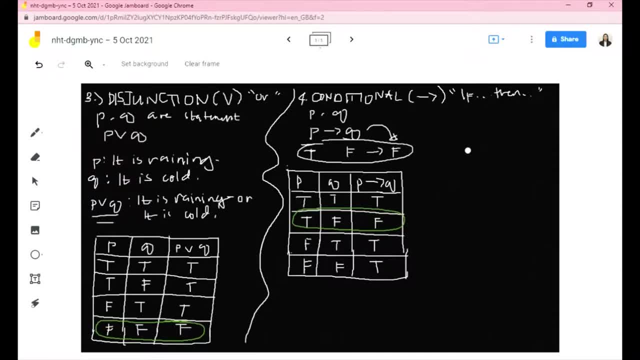 the converse, the inverse and the contrapositive. okay, so let me write in here: p implies q. this is our conditional statement. conditional statement now for the converse. we'll just have to switch the places of q and p, so from p this will become q. copy the conditional sign and we have here p. 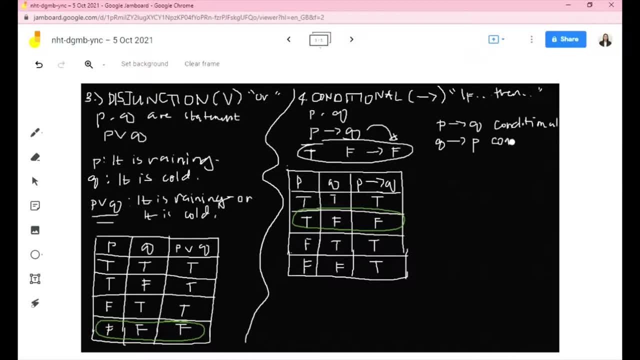 again, this is for the converse. converse. we just switch the places of q and p and we have here p and q. now we also have the inverse. what is this inverse? the inverse is simply the negation of your conditional that becomes from p. it's not p, copy the conditional sign. and q, its negation, is not q. 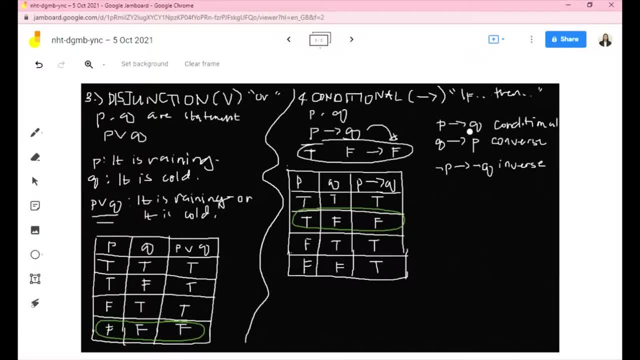 so if we have a negation for a conditional statement, then we also have a negation for the converse and that is called the contrapositive contrapositive. so from q, this will become not q, copy, the implication form or the conditional form. and we have from p, this becomes not p. okay, so again, the original form is the conditional. 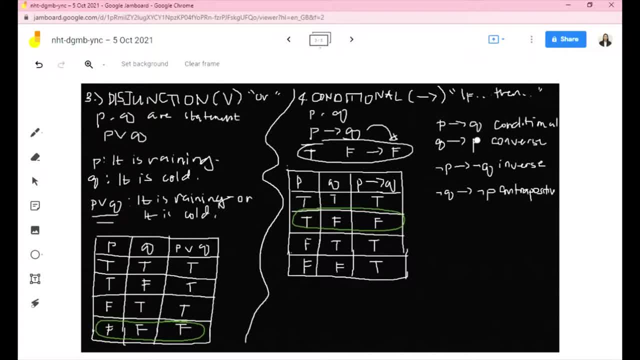 that is, p implies q. now we shift the change, or we change the places of p and q, then that becomes a converse. okay, so inverse is just the negation of your conditional statement and contrapositive is just the negation of your converse. so let's go and try to have an. 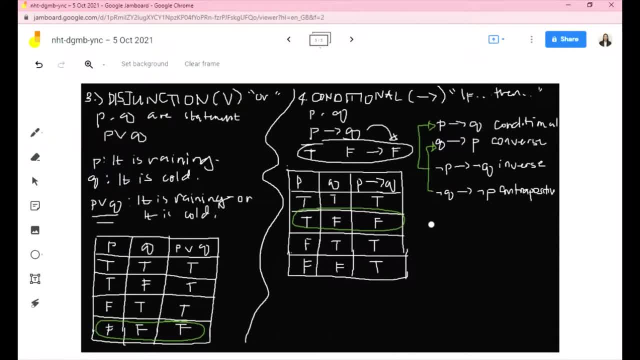 example, let's say my p. right example. let's see, or let's say that my statement p will be today is sunday and my statement q will be i will go for a walk. so let's find out the conditional form. okay, that's p implies q, so we have here. 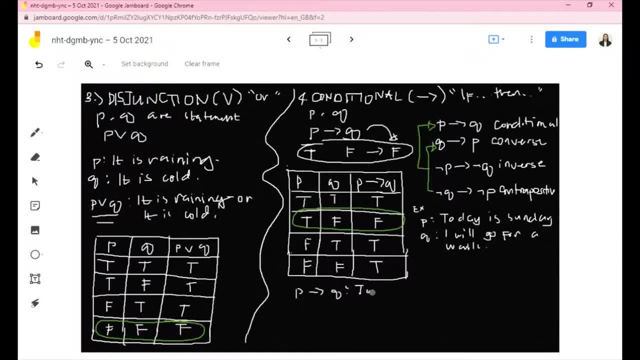 our p, that's the statement: today is sunday. oh, before we forgot, this is a conditional statement. that means we'll be using if and then then. so we'll have if if first, followed by our statement p: today is sunday. today is sunday, then i will go right, i will go for a walk. next, let's go and find the converse. so we have q implies. 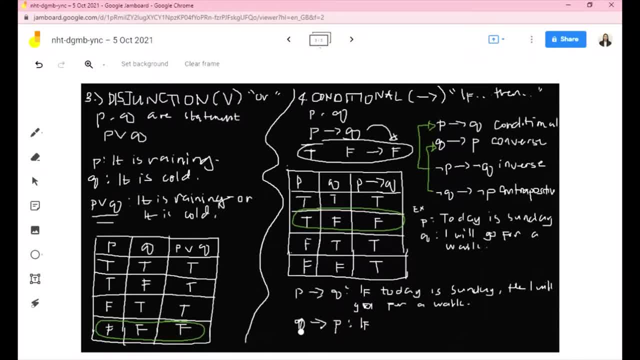 p we'll start with if, followed by our q, that is, i will go for a walk. if i will go for a walk, then today is sunday, then today is sunday now. let's have the inverse form. so for the inverse form, we can say simply that i'll just dictate this. okay, for the inverse form, or the um, the negation of your. 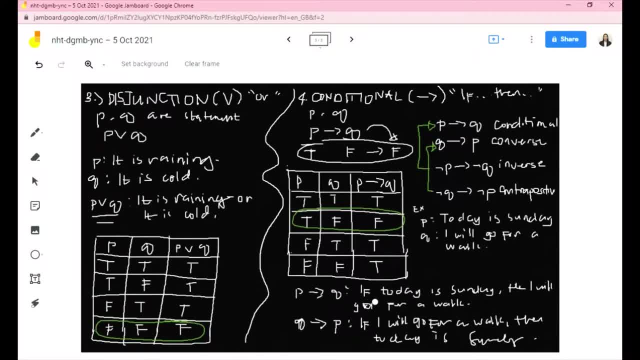 conditional. let's just say: if today is not sunday, then i will not go for a walk. okay, if today is not sunday, then i will not go for a walk. that will be your inverse. okay, if today is not sunday, then i will not go for a walk. now for the contrapositive, that will be the negation of your. 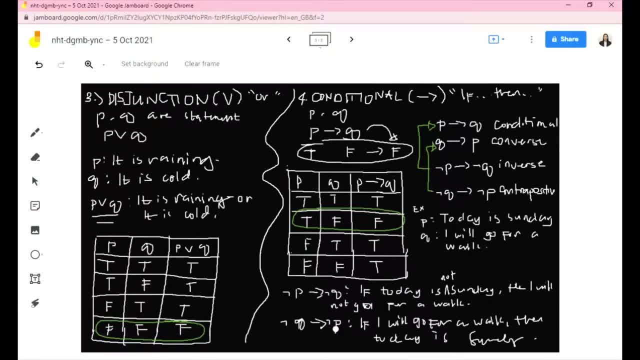 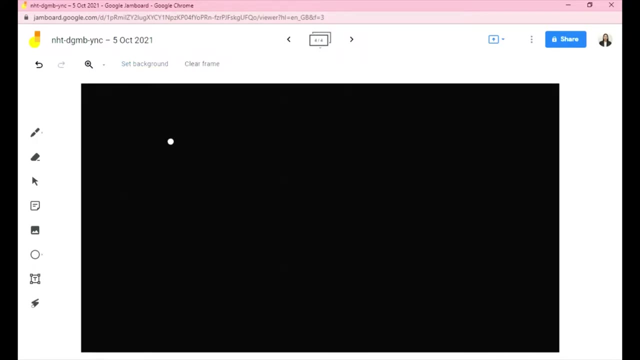 your canvas. so we have not. q implies not p. the sentence will be: if i will not go for a walk, then today is not sunday. okay, so we already have the four logical connectives. this time let's have the fifth logical connective, or the so-called biconditional. biconditional, so the biconditional. 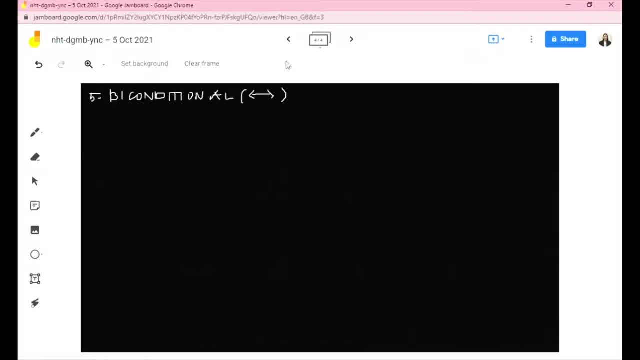 is given by this symbol and it's read as: if and only if. okay, if and only if. now let's go and continue. you suppose p and q are statements. then my common statement, using the biconditional, would be: p if and only if q. that is how we will read that: p if and only if q. so it's, it is two-way. 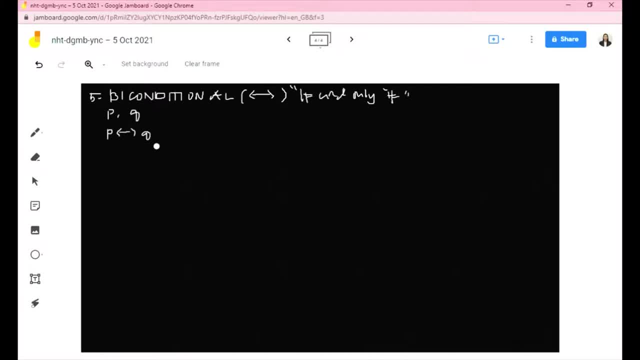 it is true, for p implies q, and it is also true for q implies p. now suppose that my statement p will be x plus 2 is equal to 5 and my statement q will be the statement x is equal to 3.. so my biconditional statement having b if and only if q will be x plus 2 equals 5, if, and only if, 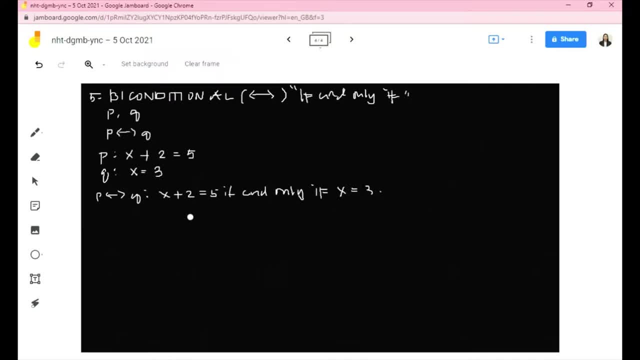 x is equal to 3.. this means that it is true for x plus 2. or if x plus 2 is equal to 5, then then x is equal to 3.. and it is also true if x is equal to 3, then x plus 2. 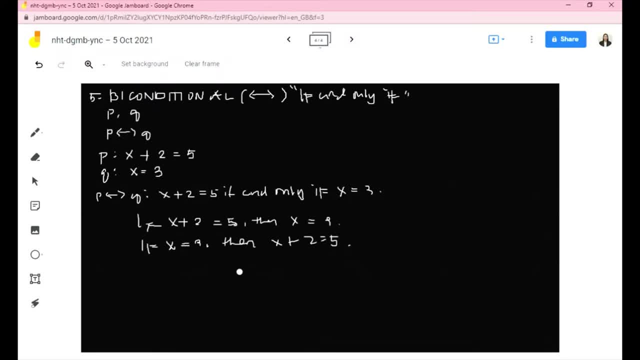 is equal to 5.. okay, for a biconditional statement. both of your propositions p and q should have the same truth values for the p, if, and only if, q to be true. a truth table. okay, truth table in here. forgive me for my drawing for my table. so we have propositional variable P. 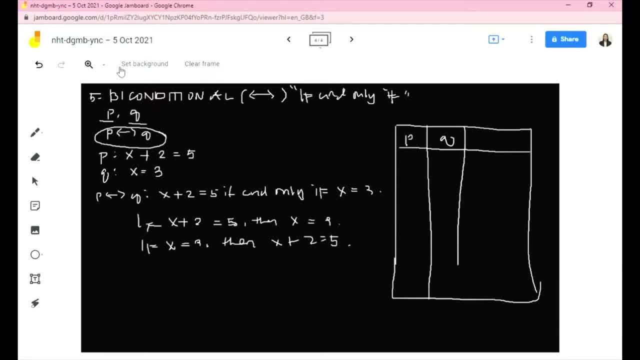 propositional variable Q, and we also have the biconditional statement P if, and only if, Q. now there are two variables involved, so we'll have four rows: one, two, three and four. the same pattern: true, true, full, false for the first column, followed by true, false, true, false. 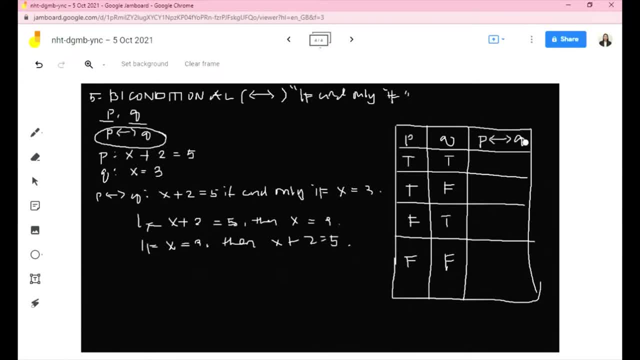 so, again, for this particular statement of a true, both of your E and Q, you should have the same same truth value: t and t if and only if t that is true. t if and only if f that is false. f if and only if t. still false if, if and only if f that is true. so, as you can notice, it can only be true. 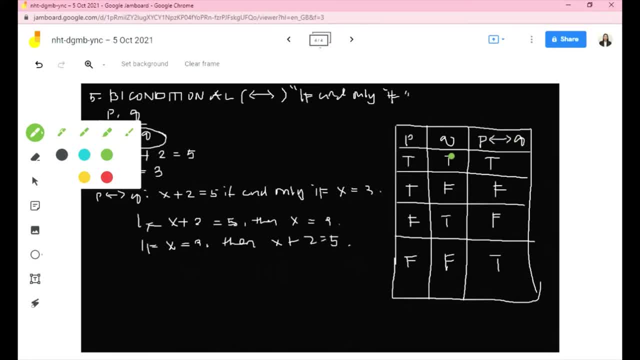 p if, and only if. q will only be true if p and q are both true or p and q are both false. in short, they pair or they have the same truth values. now, before i forgot, i want you to remember these three terms. we have the term tautology, we also have contradiction. 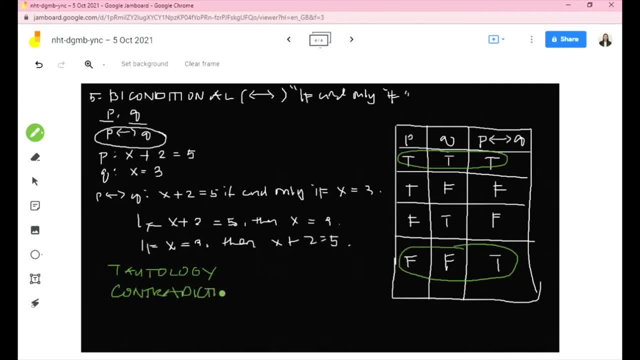 right contradiction and the other term contingency. okay, so when can we say that it is a tautology? that is, if the last part of your column for the truth table are all true, or if your conclusions are all true, then it is called a tautology. on the other hand, if all the truth, 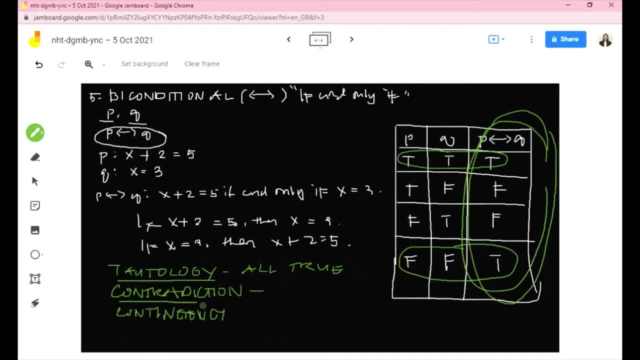 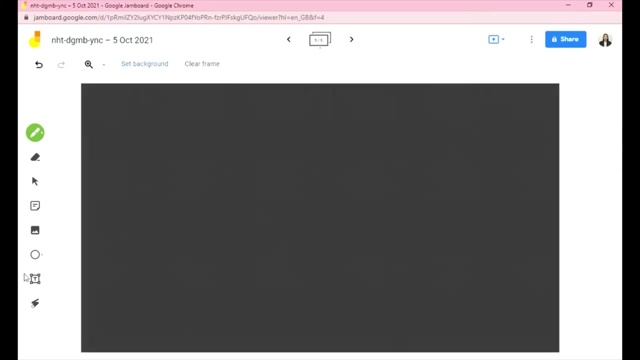 values in the last column, or all of your conclusions are false, then it is called a contradiction, right, a contradiction. but if it's neither a tautology and neither a contradiction, then it is called a contingency. okay, so let's try to construct a truth table. let's have it here. 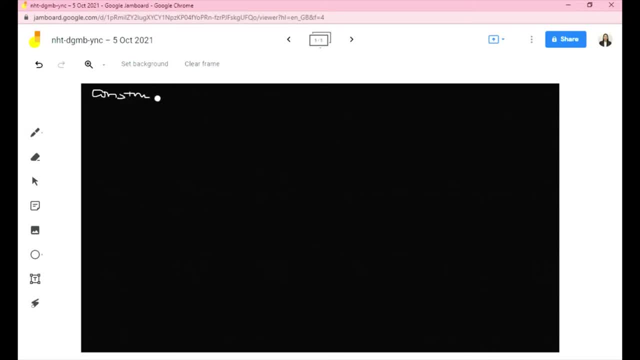 construct a truth table for construct a tb. i'll just write tb in here, tp rather, oh, i'll just go bleep it okay for a while. construct a truth table before. okay, we have here not p, and q implies not, q implies p. so we'll write down the first row first. so the first row will be your propositional variables, or? 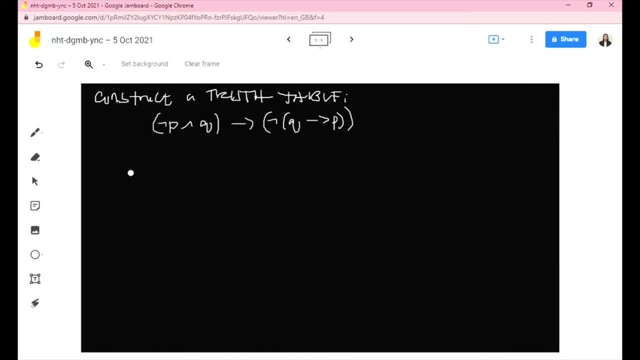 your statements, starting from the single ones, that the compound statement until the last. so let's consider, or let's rename the entire statement as a okay, so that later we won't be having troubles in writing this because it's too long. so we have the first variable, we have p. 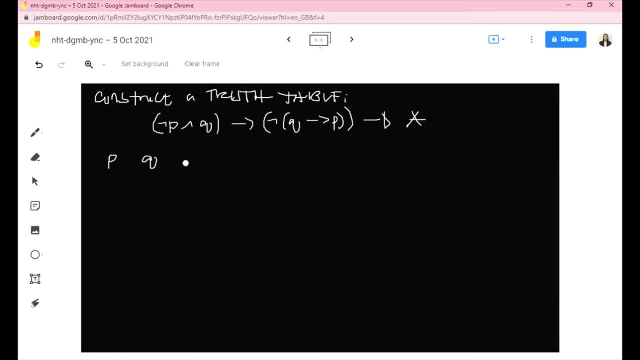 we also have q and then we have not p. take note, we have a compound statement here, not p and q. we also have the other statement here: q implies p, q implies p, and the other common statement here, not q implies p and on the last column would be this entire. 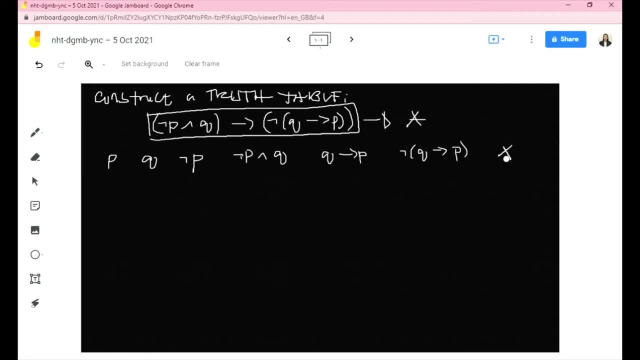 thing, or we used to represent that by using the capital letter a. so let's put a line in here, let's draw a line in here. we'll divide this by columns. okay, i'm sorry for my drawing. so still, we have two variables in here. now we'll have four rows. we'll make four rows. 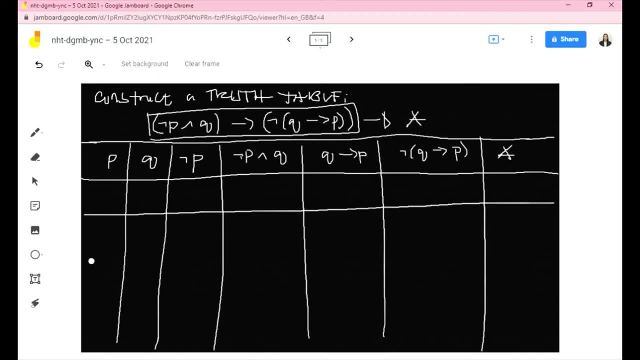 one, two, three and four. so the same pattern: true, true, false, false. but take note, you can have three or more variables, that depends on your sentence. and here we have true, false. so let's get not p. we have a p here, we have not p here. that means we'll taking the negation of our p. 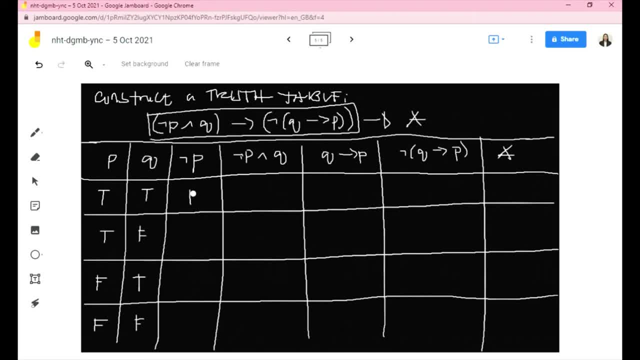 so if my p is true, my not p will be false. if my p is true, my not p will be false. if my p is false, my not p will be true. if my is false, my not p will be true. true as well. now let's have not p and q, so let's go not p and q. this particular column in here and this: 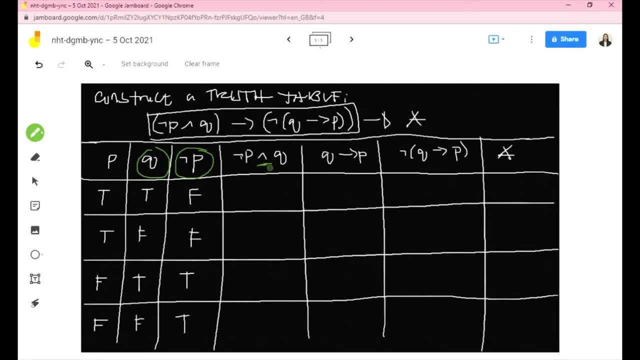 particular column in here we have, and that means both of them should have the same truth values, or both of them should be true. okay, both of them should be true. now let me remove the circle. not p and not q, not q, rather not p and q. so we have f and t that is f, f and f that is f. 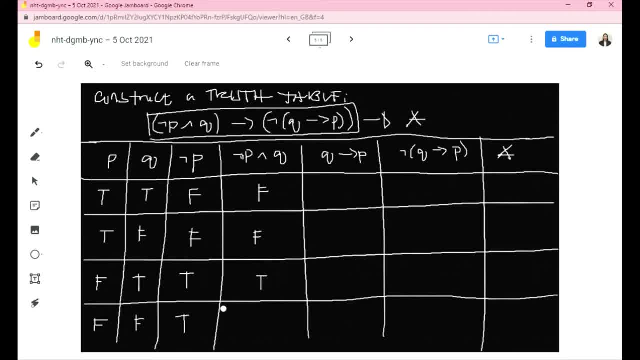 t and t- that is true. t and f- that is still false. now let's go for the. q implies p, so we'll start from q to p. this is implication or conditional statement. that means there is only one way to make it false, and that is when your first proposition or your 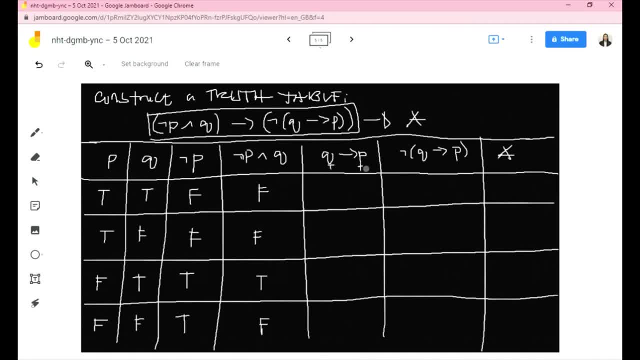 antecedent is true, but your consequent is false, So in that case it will be false. Now let's continue. Q implies B, So T implies T, That is T. F implies D, That is T. T implies F, That is F. F implies F, That is T. Now let's have not. Q implies B, So the negation. 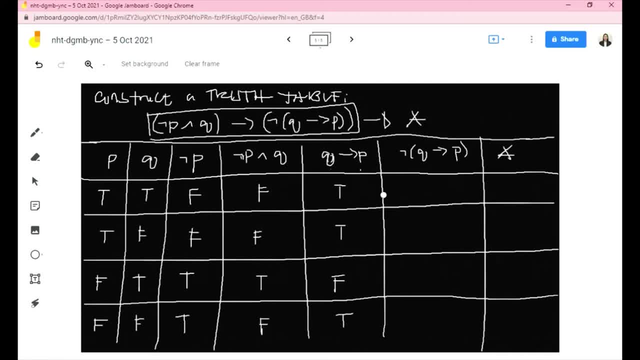 of this entire column: Negation of T- That is false. T, That's false. False That becomes true. True, That becomes false. Now we are down to our final statement. So we have not. P and Q implies Right. So we'll be using this one, Not P and Q implies this. 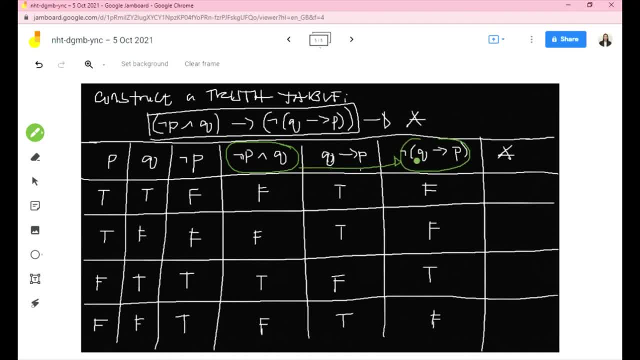 statement Not Q implies P, So we'll start here. So implication again: This can only be false. if your P or the first proposition or the first Santa Claus statement is true, your antecedent is true, but your consequence is false, then you'll have 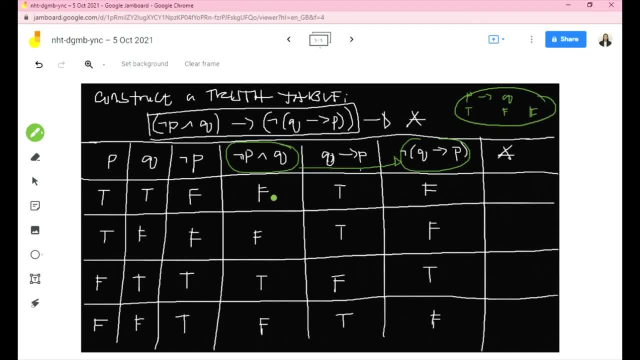 false in here. This will be the only case. So let's begin. F implies F that is T. F implies F that is T. T implies T that is T. F implies F that is still T. So you see our conclusions. 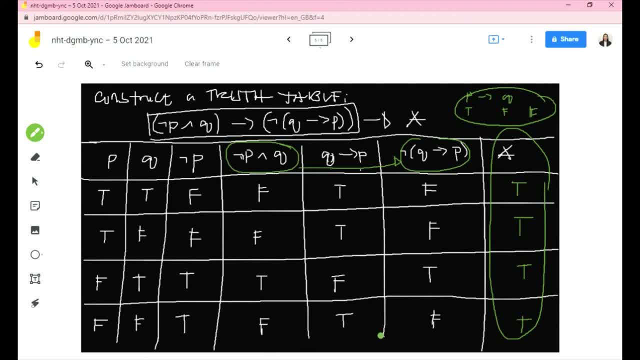 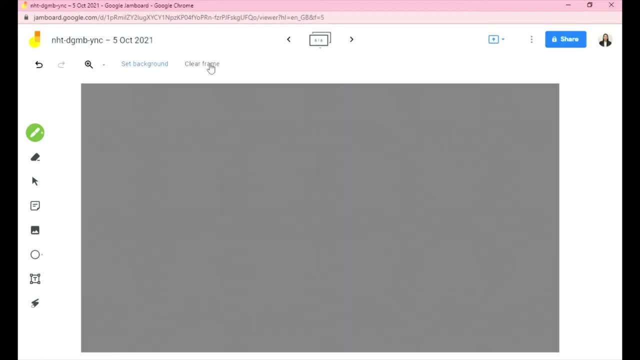 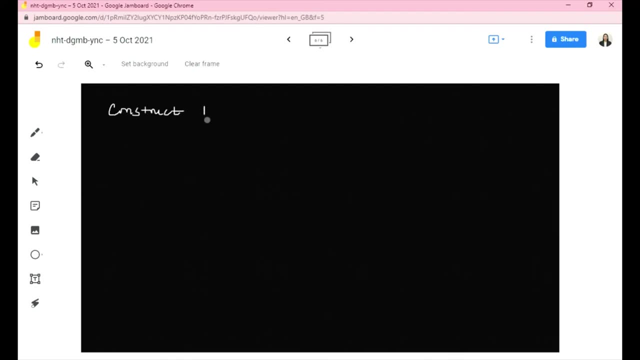 are all true, then that means we can consider this one as a tautology. Okay, Now let's have another example. Let's construct the truth table, or construct the truth table of not P and P. So in this case we only have two variables: that from 2n that becomes 2 raised to 1.. So we 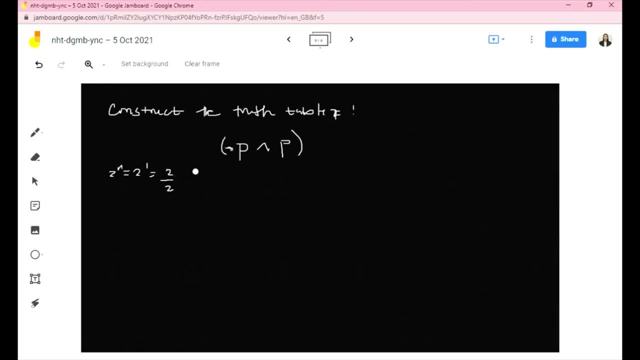 have 2.. 2 divided by 2, then we'll have one true, followed by one false, as our pattern, and we only have two rows in here. So let's draw the truth table. Okay, We have P, We have not P and we have our final statement: not P and P. No, we only have two rows in here. 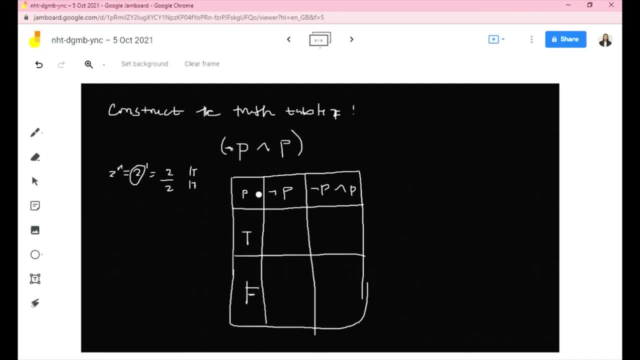 1T- 1F. So if my P is T, my not P will be F. If my P is F, my not P will be T. Now let's have the conjunction of not P and P, So it uses: 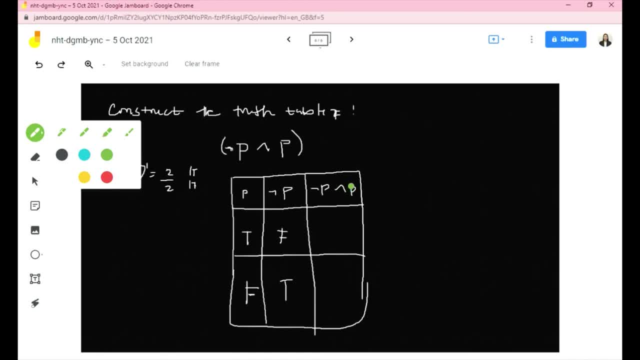 and it uses conjunction. This means both, not P and P, should be true. Now we have T and F, that is F. We have F and T, that is still F, So all of our conclusions are false. then that means it is a contradiction. Now, if it's neither a contradiction nor a tautology, then it's considered. 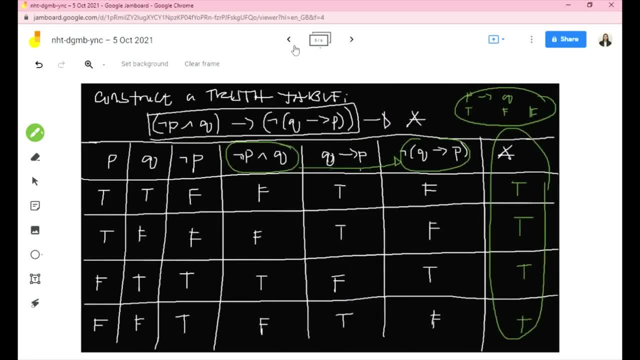 as a contradiction. I hope I made this clear Now. if you have questions, feel free to ask me. Okay, Goodbye, and God bless us all.